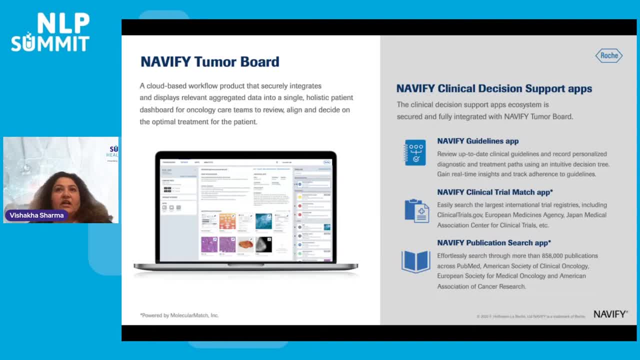 by securely integrating and aggregating relevant patient data, It enables multidisciplinary teams to work together more effectively, virtually or in person. The software has built-in analytics reporting capability to support metrics essential for accreditation and quality measures. In addition, clinical decision support apps are fully integrated with Navify Tumor Board to provide. 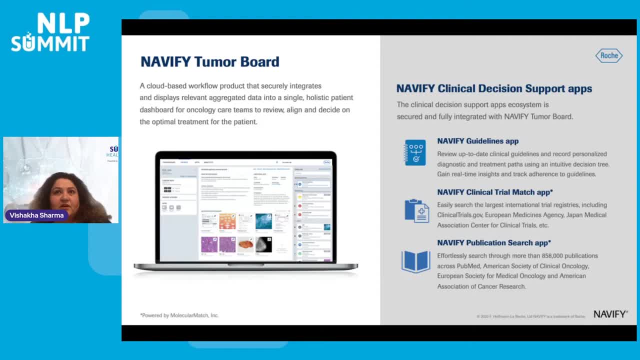 personalized clinical trial and publication search results. Clinicians can also access digitized national or comprehensive cancer network NCCN guidelines to find and review guideline recommendations based on patients' clinical information. pin relevant guideline recommendations to a patient case for an upcoming multidisciplinary team meeting. 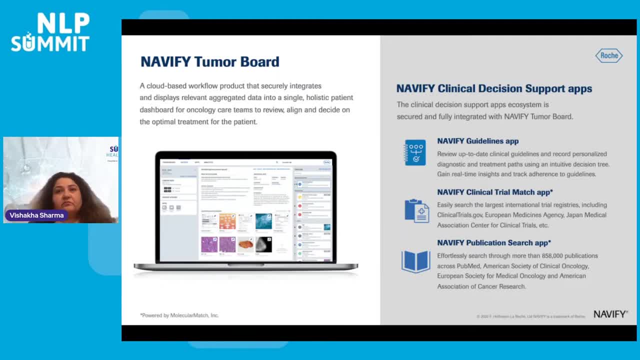 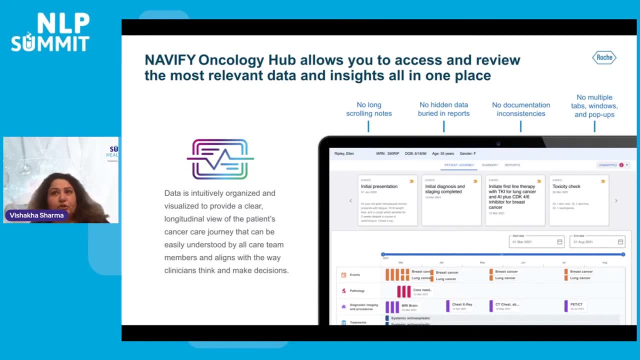 or print them for patient and payers. Our secondary portfolio is Navify Oncology Hub. that is a clinical workflow decision support platform that supports clinical trials and decision support solution designed to simplify and improve day-to-day clinical decision making and care coordination across the oncology care continuum. It does so by aggregating and 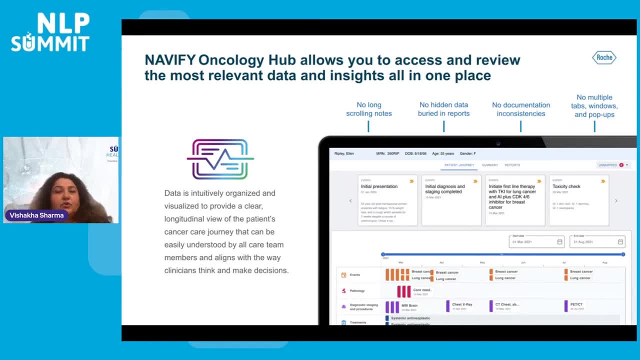 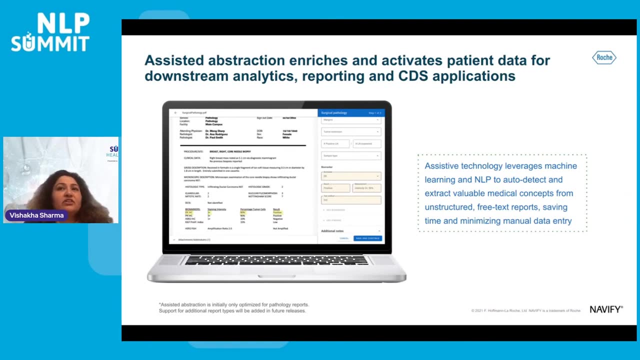 organizing fragmented data, providing an intuitive longitudinal view of the patient's entire care journey that can be accessed and used by all members of the oncology care team. So unstructured data from the free text reports are not available for quick consumption at the point of care and are inaccessible for advanced decision support analytics or quality reporting. 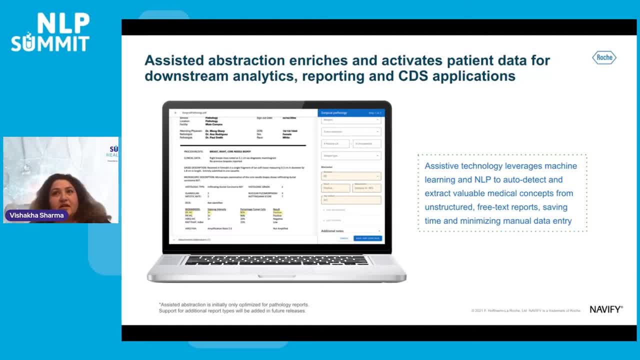 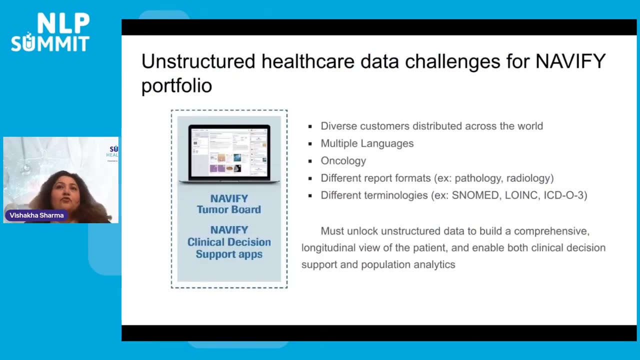 Navify abstraction, leverages, natural language processing and machine learning to auto-detect medical concepts and translate free text into data that is structured and enriched, while reducing the burden of manual data entry. So for a cancer patient, a large number of data points get generated along their journey. 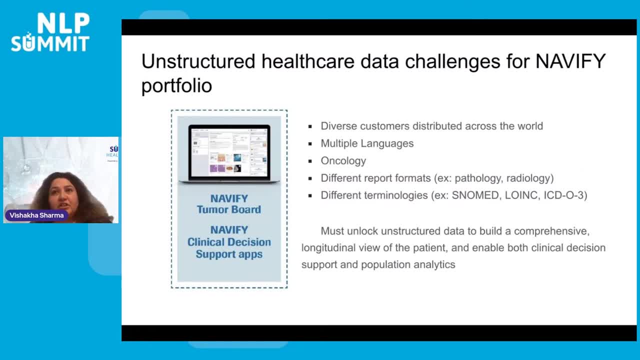 for example, genomics, pathology, radiology, their clinical data. The goal here is to investigate through the complexity of patient's journey and generate a longitudinal view by unlocking these data sources And, for a more comprehensive view, unlocking unstructured data is very important. 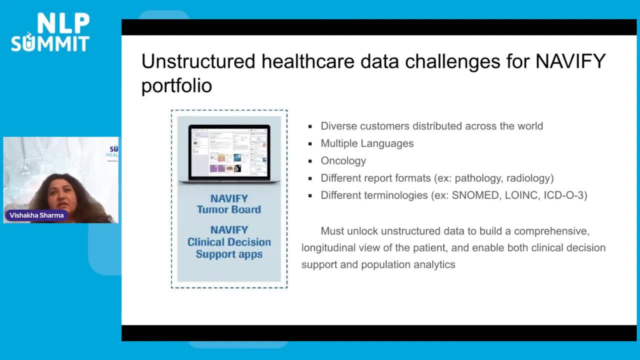 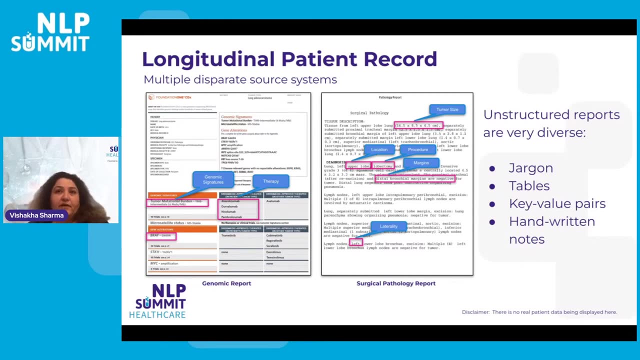 because a lot of time this has diagnosis and treatment information. These data allow us to do clinical decision support and population analytics. One of the major challenges in healthcare is to consolidate these unstructured data like genomic signatures, therapy information, size of tumor, etc. 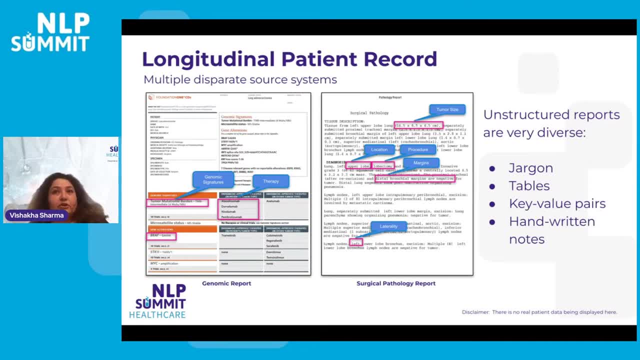 from different sources like genomic, pathology or radiology reports, And these reports are very diverse. they may have something different, structures like jargon tables, p-value pairs and so on. So if you're interested in learning these results, please feel free to write us an email at. 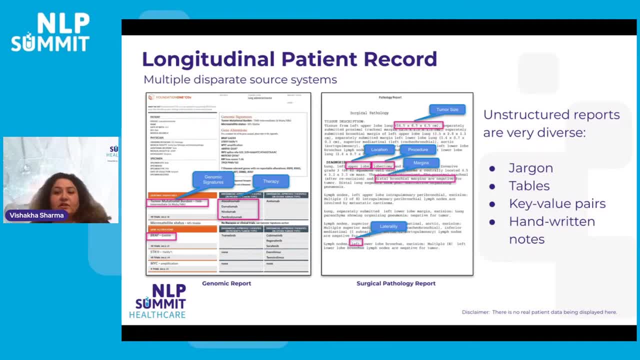 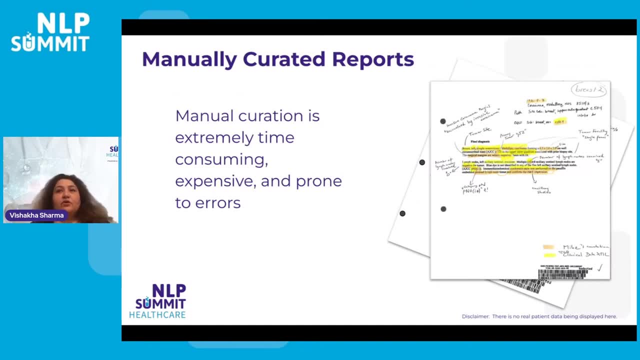 http//theleoadvnet, or check out our linked link in the description box: pairs, handwritten notes, etc. So in a lot of cases when a sample report gets reviewed, for example by a pathologist, it looks something like this: And how many of you have seen something? 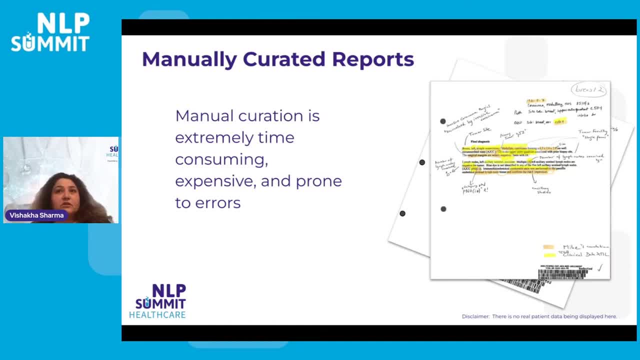 like this Because it's a handwritten text And if you read closely you can see there are talking about tumor size, tumor staging, ICD codes and a bunch of other things. All of these annotations make this report extremely valuable, But the challenge is: how do we extract all of this? 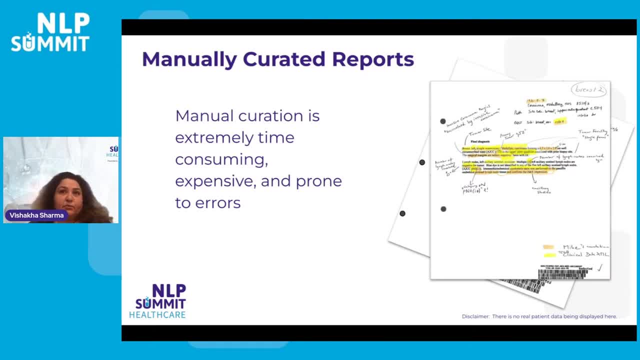 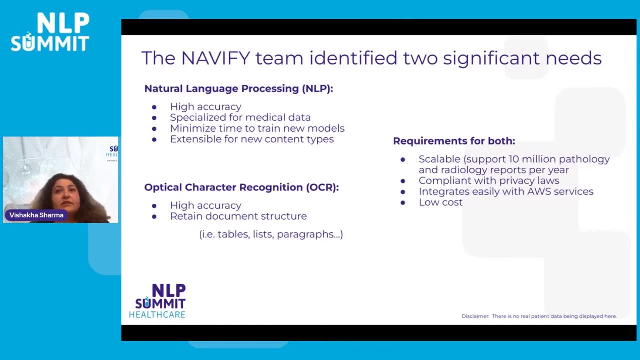 valuable information to enable clinical decision support. So it is quite clear after looking at these reports that, along with NLP, we will need optical character recognition to efficiently extract information. So now, what is optical character recognition? Optical character recognition is a recognition of printed or 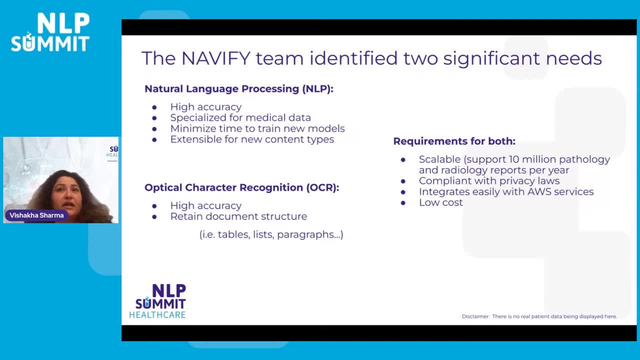 written text. We need natural language processing with high accuracy, specialized for medical data, with minimized time to train the models that can be extended for new content types. We need optical character recognition with high accuracy and ability to retain document structure like tables, lists and paragraphs. So we had a bunch of requirements from tools and services. 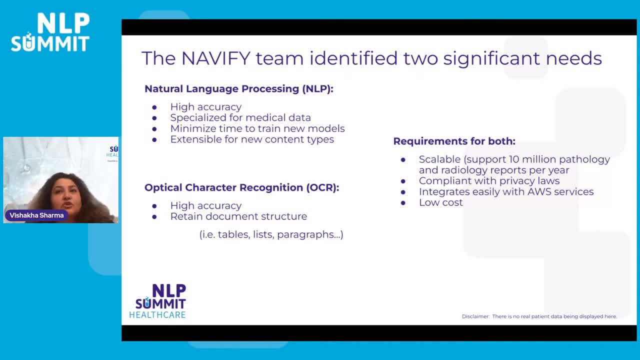 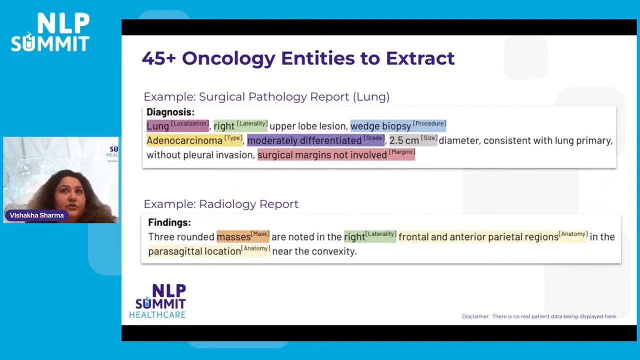 that could help us achieve this task or need. So the first step is to identify the main entities from the domain specific documents. These entities are highly specific to the use cases, So health care data is extremely heterogeneous and complex and requires high quality labeling data. 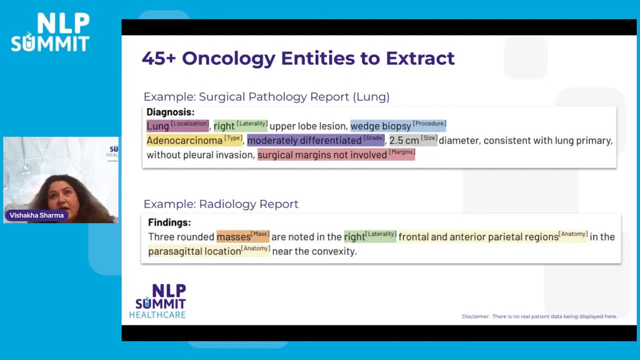 and domain expertise and that can be very expensive and time consuming for any organization. So at Roche we have extracted more than 45 oncology entities from pathology and radiology reports. Here are a few examples of surgical pathology report and a radiology report. 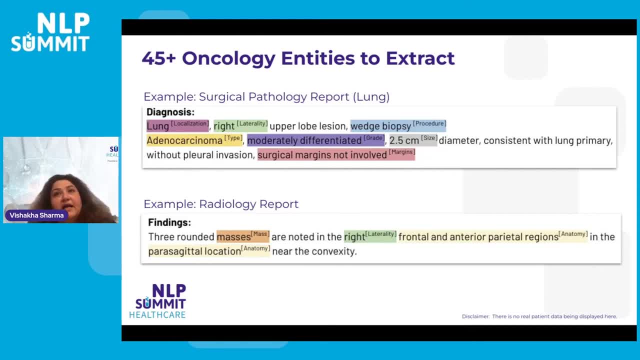 from patients diagnosed with lung cancer. So the highlighted text shows the entities of interest and its associated labels. The first example shows our diagnostic information of a lung patient: lung right upper lobe lesion VEG biopsy: adenocarcinoma moderately differentiated. 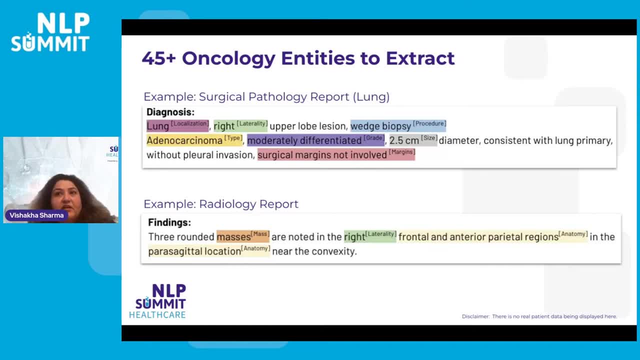 Their lung is the location and right is the laterality and VEG biopsy is the procedure and 2.5 centimeter is the size of the tumor And it says surgical margins are not involved. The second example shows the findings of a lung patient. 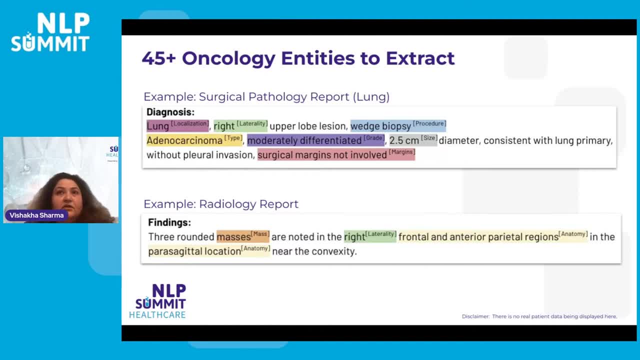 like three rounded masses are noted in the right frontal of anterior parietal regions, in the paracegital location near the convexity. So in this sentence three masses are found for the patient and we label masses as mass. right is the laterality. 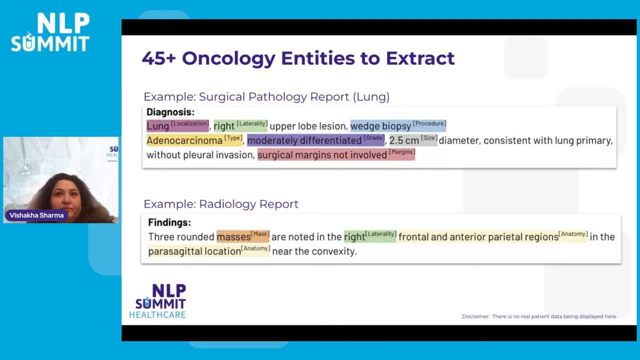 frontal and anterior parietal regions are the anatomy. So if you see this example, you see different types of labels and it's associated values and mentions of cancer type localization procedures And our approach has been, as first step, categorizing the content broadly as possible. 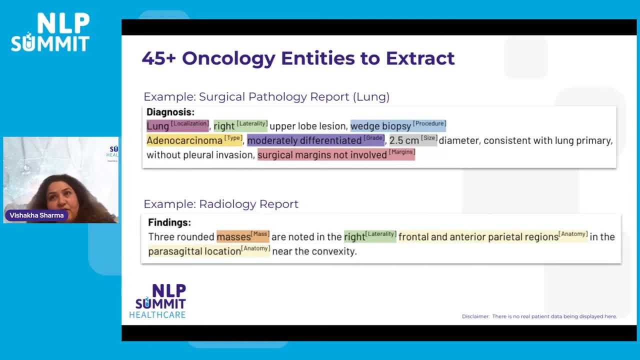 And this helps us achieve high recall with entity extraction And we then, in the next term, drill down to achieving high precision by mapping these entities to standard concepts And towards the end, we try to form relationships, to extract the proper relationship context from these complex healthcare sentences. 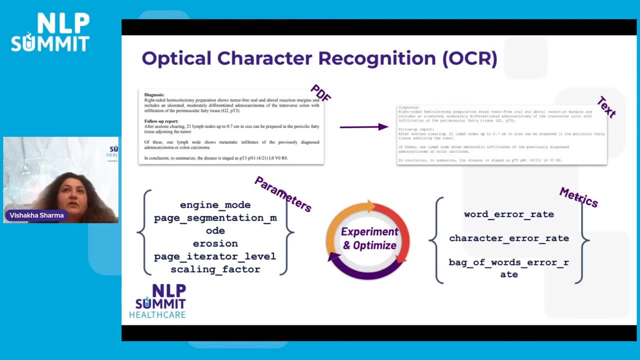 So before I discuss how I evaluated optical character recognition, I want to reiterate basically optical character recognition stands for basically it is a technique that is used to convert document images to machine readable text. So goal here has been, as you can imagine, to make sure we can. 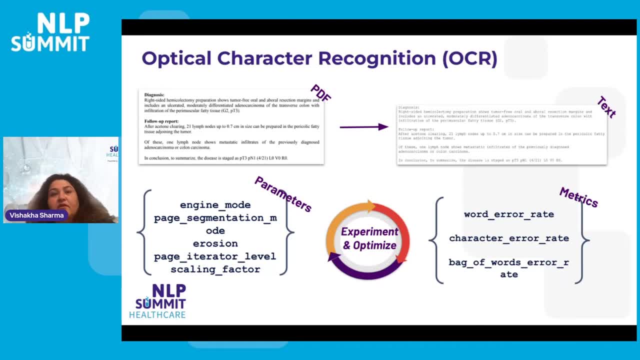 consistently convert the PDF with text and image layers of these pathology, genomics and radiology documents into human readable text format. To evaluate the performance of this OCR system, we used a combination of matrix, starting with character error rate, which is nothing but the minimum number of operations. 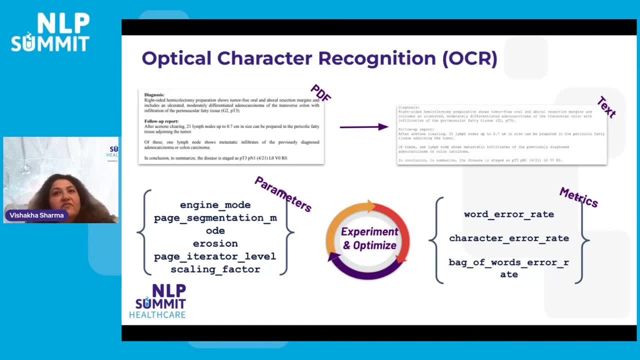 required to transform reference to output. Then we evaluated based on the word error rate, which is the number of words substituated, deleted or inserted from reference to output. Evaluating word error rate poses some challenges, like spacing and length of word sequences. To overcome this we use the bag of words error rate. 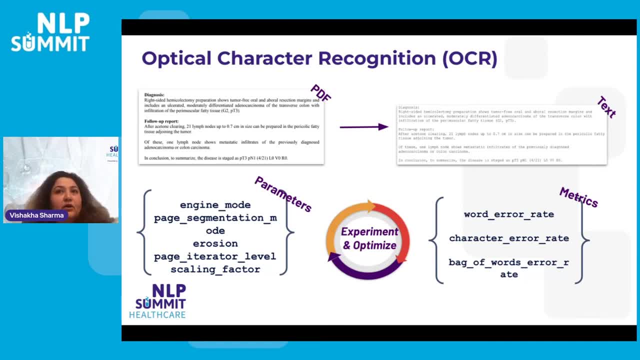 where, instead of looking of words, you look at the bag of words. Each of these matrix were measured against a bunch of OCR system parameters, like if the document is a text or an image. So what basically we have? we have in OCR system. 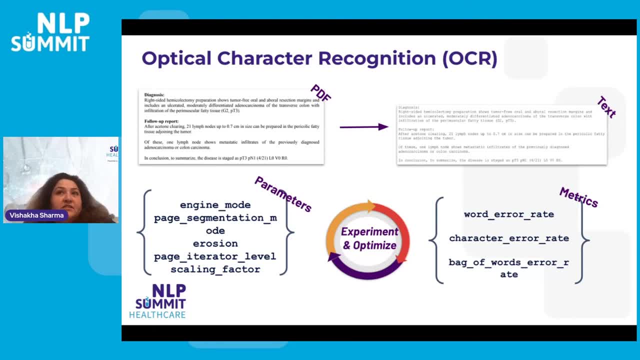 we have a parameter called as engine mode or the page segmentation mode, which tells the system if the document has a single character or a block of text, or tables, et cetera. And third is erosion or scaling factor. So overall, on the matrix, against our ground truth. 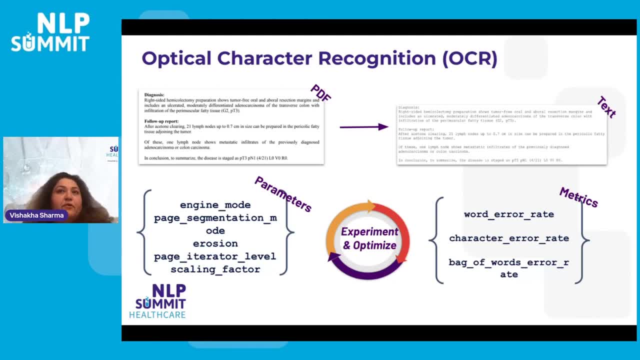 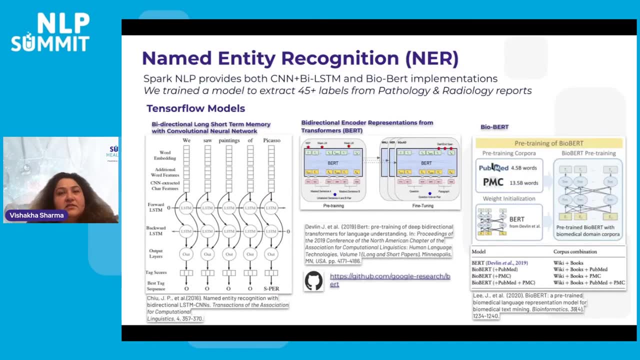 we landed on a set of value of our parameters that performed well on our data. So our next task after optical character recognition is named entity recognition And in simple words it's basically entity extraction and is a subtask of information extraction that seeks to locate and classify named entity mentions. 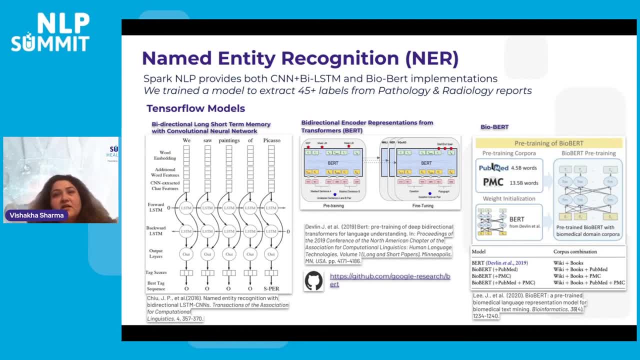 in unstructured text into predefined categories, such as tumor site, primary tumor, et cetera. So this is what the current state of these deep learning models are. So if you look at on the left hand side, the first is basically CNN by LSTM. 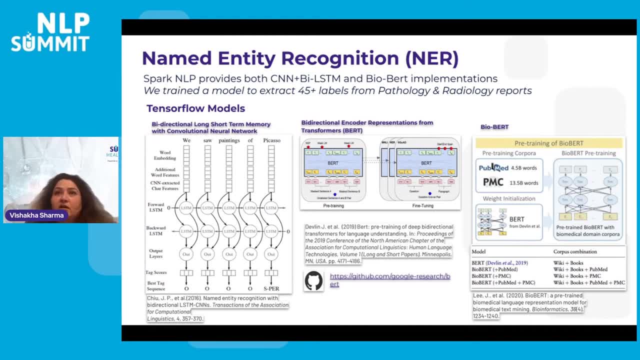 Which is a novel neural network architecture that automatically detects word and character level features using a hybrid bi-directional LSTM and convolutional neural network architecture, eliminating the need for most feature engineering, And this work was published by Jason Chu in 2015.. The second is BERT. 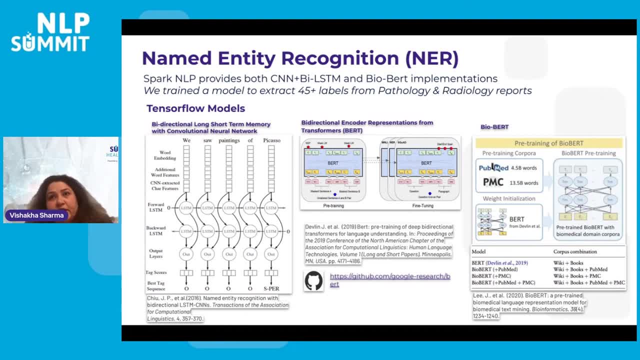 The BERT stands for bi-directional encoder representation from transformers. Unlike recent language representation models, BERT is designed to pre-train deep bi-directional representations from unlabeled text by jointly conditioning on both left and right context in all layers, And this work was published by Li in 2019.. 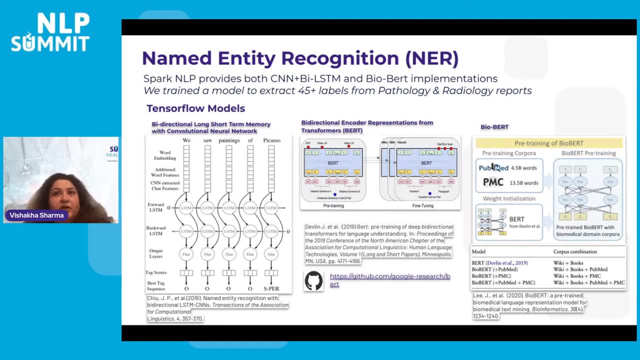 BioBERT is, I will say, the first domain-specific BERT-based model pre-trained on biomedical domain, corpora, which is primarily PubMed abstract, And this work was published by Li in 2019.. Spark NLP provides both convolution neural networks. 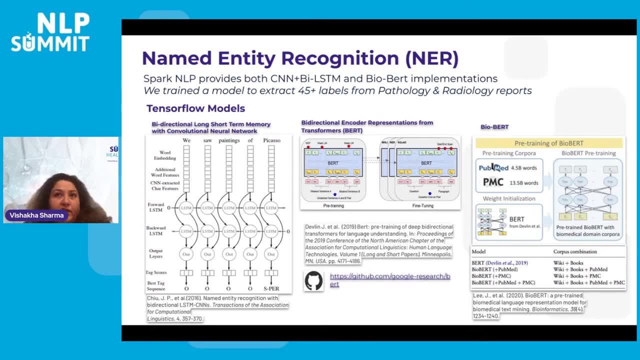 BiLSTM and BioBERT implementations. We train a CNN BiLSTM model to extract these 45 plus entities from pathology and radiology reports using Spark NLP, And this work was published by Li in 2019.. And this work was published by Li in 2019.. 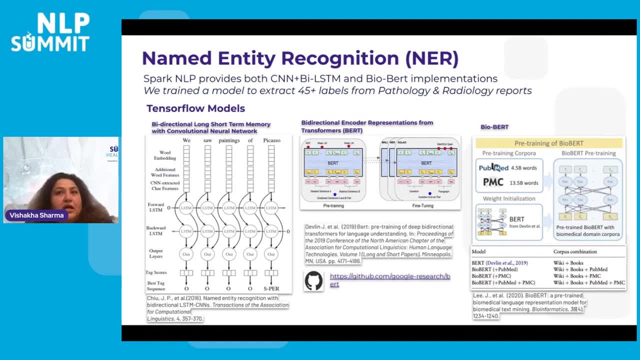 Spark NLP provides both convolution neural networks, BiLSTM and Biobert implementations, Right Spark NLP For relationship extraction. they have a multi-layer perceptron neural network model that we are using to extract the relationships from these complex reports. 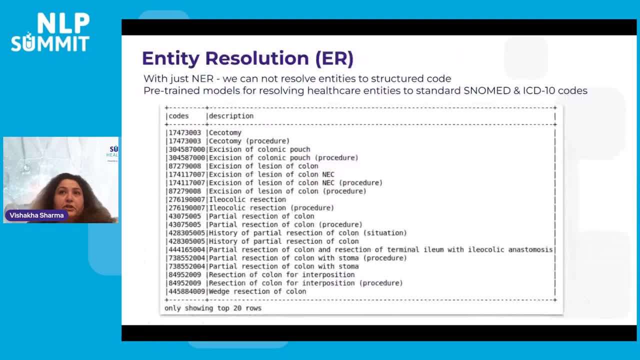 So I talked about named entity recognition, optical corrective recognition and briefly on relationship extraction. But with just these approaches we cannot structure, un-structure text. So what is entity resolution? So entity resolution means removing duplicates, normalizing data, disambiguating records, 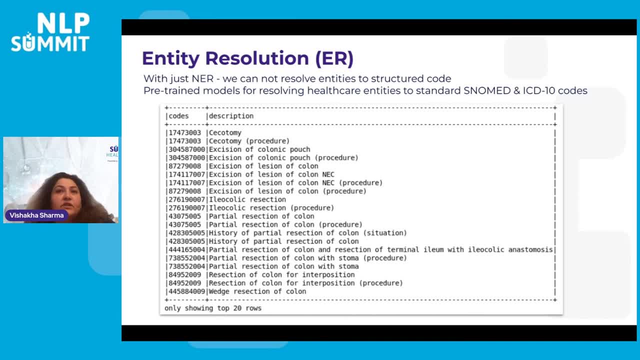 that correspond to real-world entities across and within data sets. We have been looking into approaches which combine clinical embeddings and named entity resolution to pick appropriate terminology, concepts similar to named entity recognition, entity resolution models and data sets, And we have found that the most common approaches 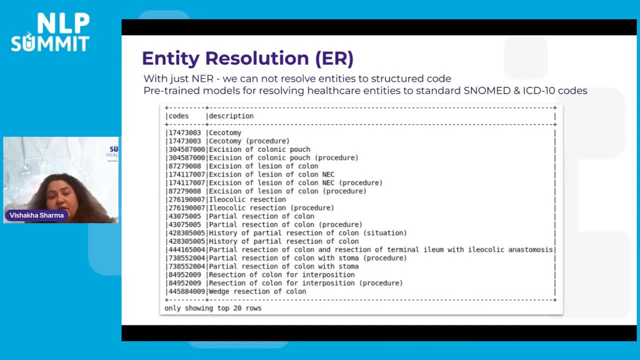 are for terminology or ontology like ICD-10, RxNorm, SNOMED, et cetera, For example for tumor staging information, for TNM values- we follow AJCC standards Right- And for something like drug-related entities. 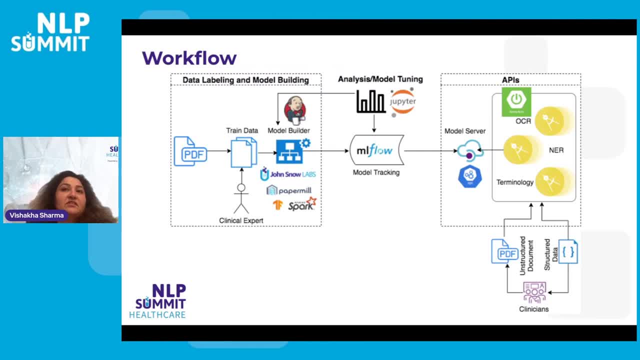 we follow RxNorm. So now that I have discussed the techniques that I used, let's talk about the process. So what we'll see here: The first step is to understand the model. So we have a model that we have adapted. On the left-hand side, I show how the model is built. 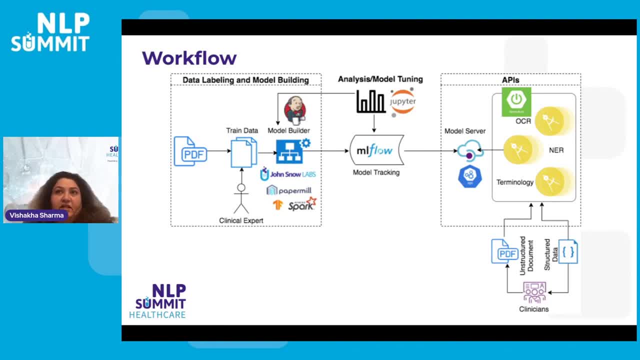 And on the right side we see how the model is served and consumed. There are many elements here for building the models in an automated manner. We stuck with old-fashioned Jenkins, which we use for orchestration. Another choice we made was to stick. 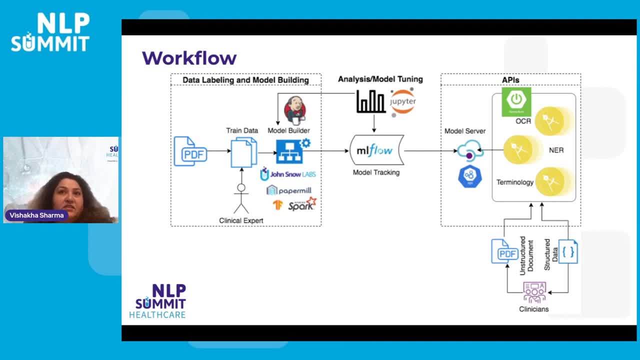 with Jupyter for exploratory data analysis and even run it in the pipeline. So we have a model called PaperML. Our NER and OCR implementation is Spark NLP based. We use MLflow to track performance of each run, along with recording the artifacts. 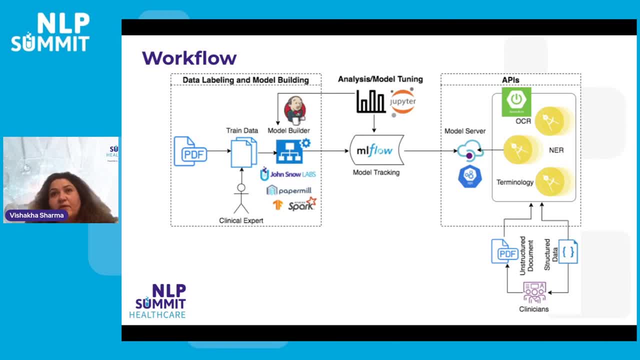 This gives us the ability to compare, pull and deploy artifacts from any run. We deploy the latest model that reaches threshold performance as APIs which then can be consumed by downstream applications. This is our sandbox. Getting to product is a little more manual. 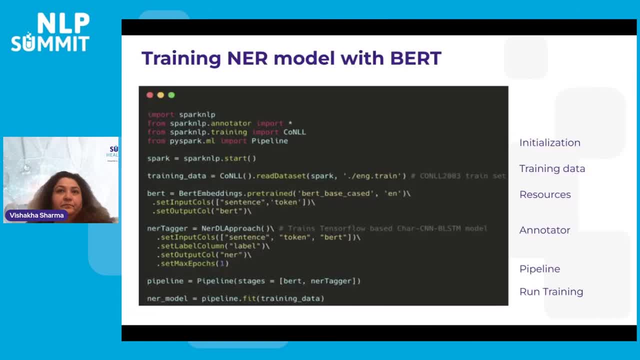 but it's a lot of work And it's a lot of work to build the NER in a highly-regulated environment. You might wonder how much code it would take we have to write to build a NER model with embeddings. It is actually just a few lines with Spark NLP.